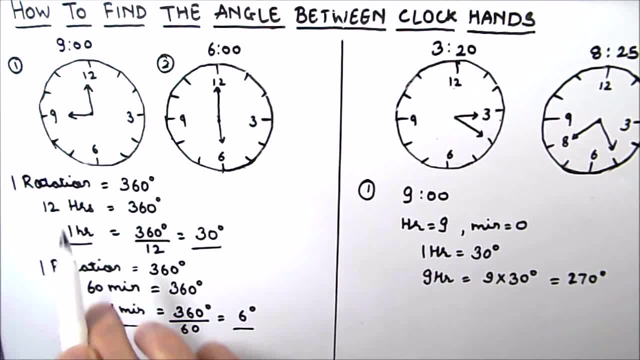 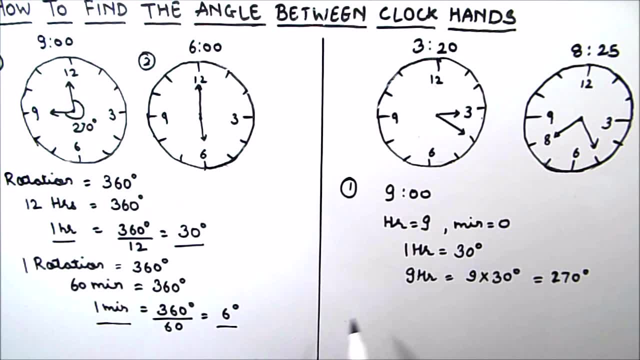 270 degrees. So here this is 9 o'clock angle made. is this one which is 270 degrees In our next example, where the time is 6 o'clock, so the hour hand is at 6, so hours is 6 and minute hand. so we can find the angle for 6 hours as 6 times 30 degrees, which is equal. 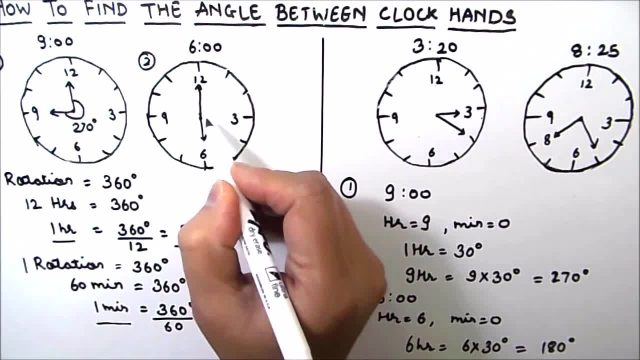 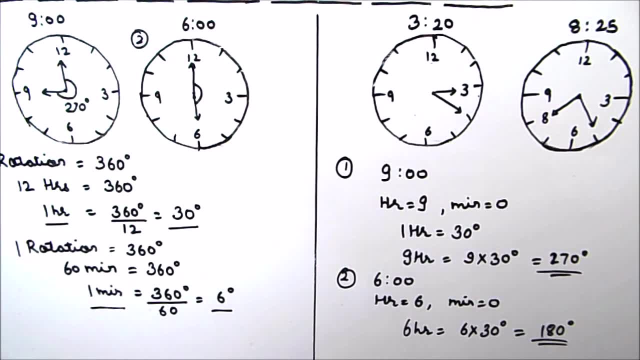 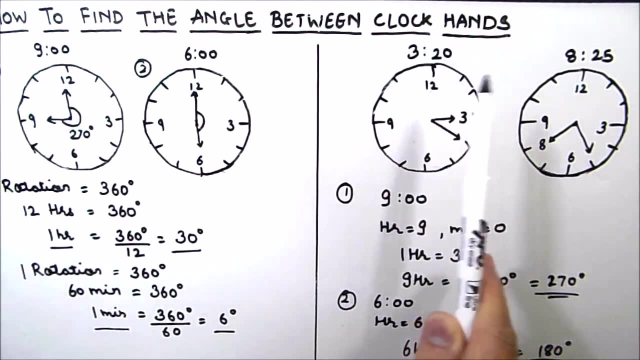 to 1 hour. So here we see the angle made. so these are the two examples in which the minutes hand is at 12 or we can say is angle made by the minute hand is 0 degree. Now let's try few more examples where the time is in hours and minutes, both. 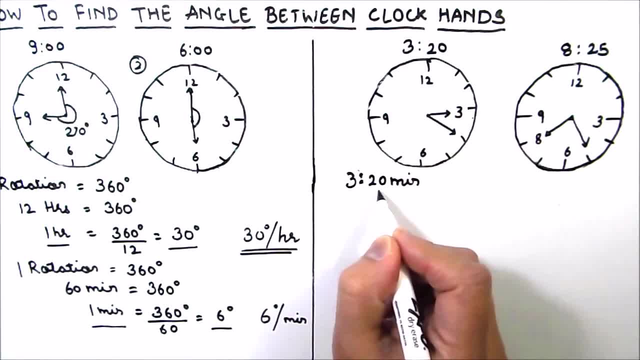 Now let's consider an example where the time given is 3 hours 20 minutes. For this calculation, we need to understand that the hour hand also moves for 20 minutes. It's not only the minute hand which moves, it also the hour hands which move for 20 minutes. 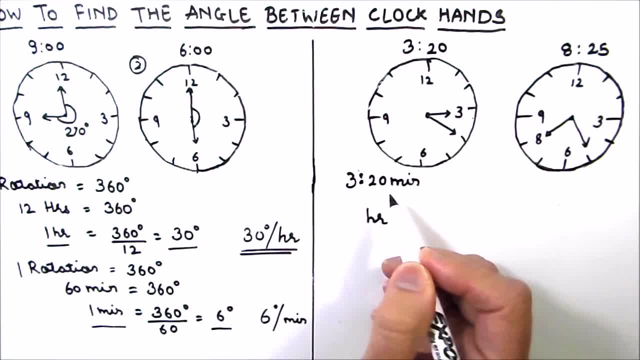 So we have to consider the movement of both the hands for calculation of hour angle. So the formula for this is: hour plus minute divided by 60 degrees, because one rotation is 60 minutes, Multiply by 30, because it is making an angle of 30 degrees per hour. So here, as our time is 3.20.. So we can calculate the angle for hour. So here, as our time is 3.20.. So we can calculate the angle for hour. So here, as our time is 3.20.. 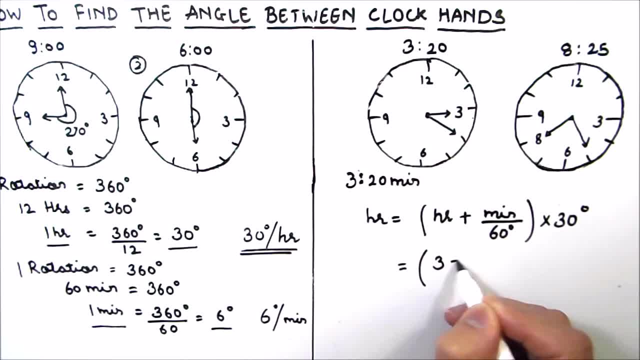 So we will write 3 hours, 3 full hours, plus 20 minutes, which is part of the 60 minutes multiply by 30. So this will become 3 plus 1 by 3 multiply by 30, which is equal to 3 times 3 is 9 plus. 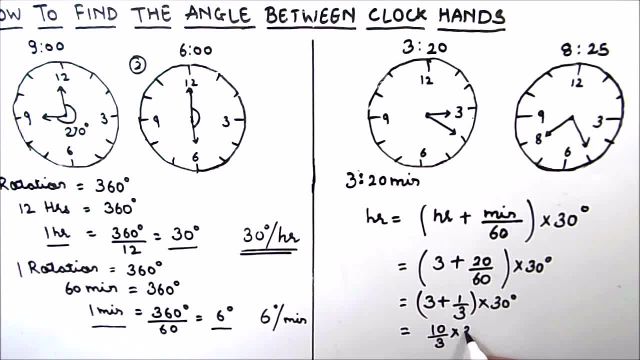 1 is 10 by 3. multiply by 30, which gives us This is 3 times 10. so 10 times 10 degrees is 100 degrees. So our hand will make an angle of 100 degrees. Now we have to consider the minute hand's angle too. 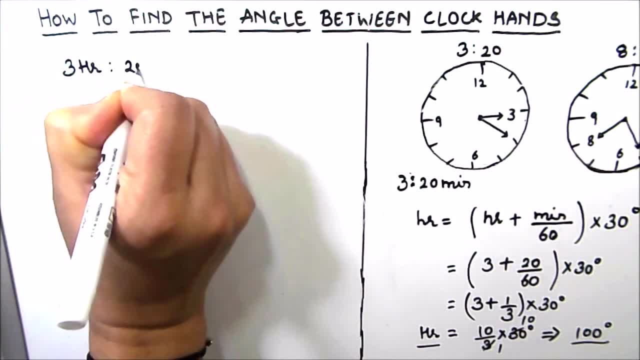 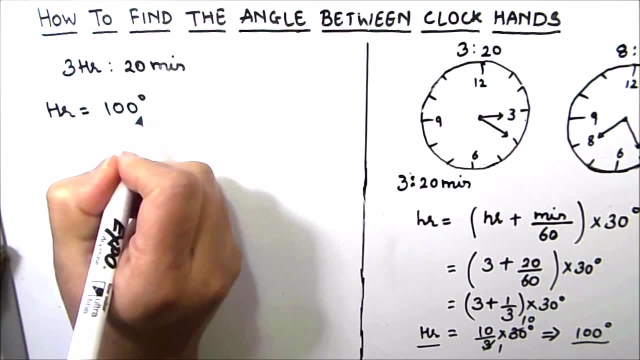 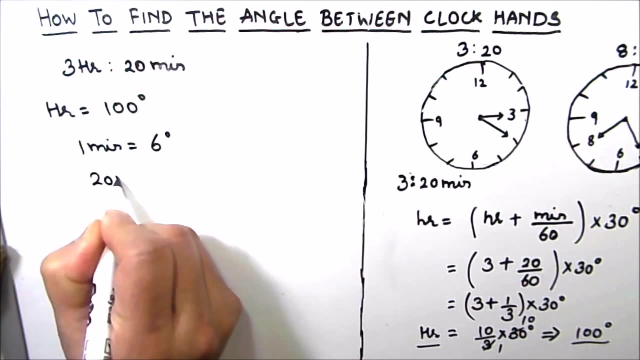 So our time given is 3 hours 20 minutes hour. we calculated as 100 degrees. Now we have to calculate the angle made by minute's hand. So one minute it is making an angle of 6 degrees. So for 20 minutes the angle will be 20 multiplied by 6 degrees, which is equal to 120 degrees. 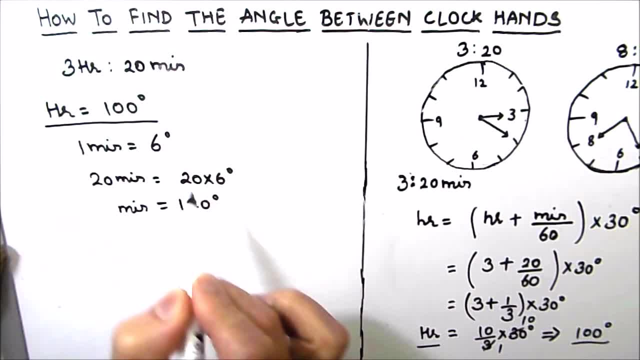 So this is for minutes. We have hour angle, we have minute angle. Now to find the final angle between the hands of the clock, we have to take the absolute value of the difference between angle made by hour hand and angle made by the minute hand. 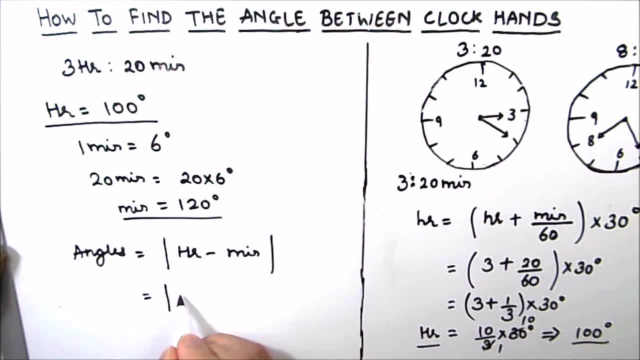 So absolute value of hour hand angle is 100.. 100 degrees minus minute hand is 120 degrees. We are taking the absolute value because the angle will always be a positive angle. So 100 minus 120 is 20 degrees. So the angle made between the hands of the clock when the time is 3 hours 20 minutes. 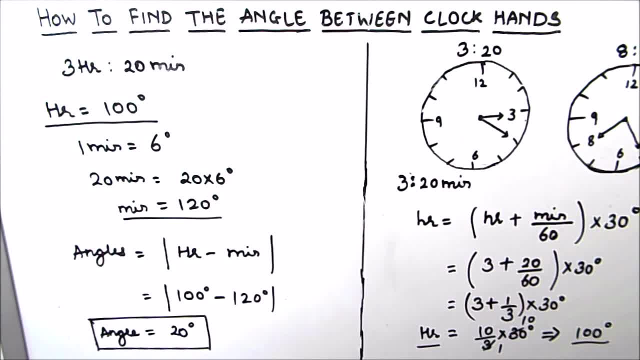 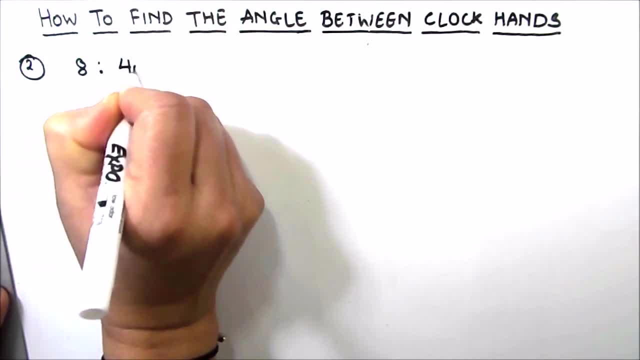 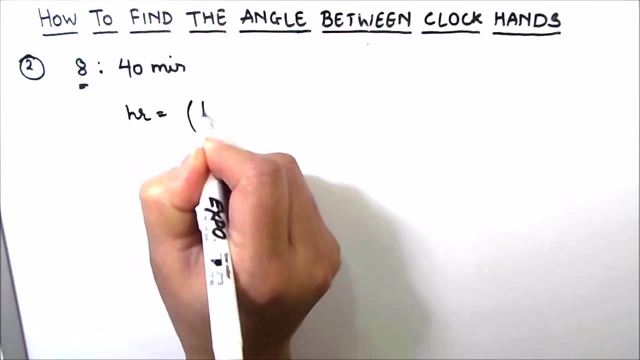 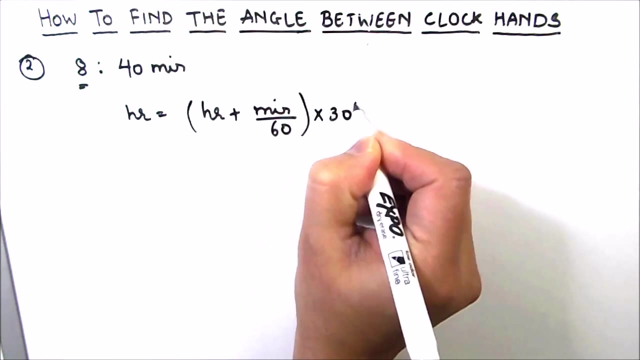 is 20 degrees. Let's try one more example of this kind so the calculation is more clear to us. So in this case We are taking time as 8 hours 40 minutes. First we will find the angle for hours. So the angle for hours is hour plus minute by 60, multiplied by 30 degrees. 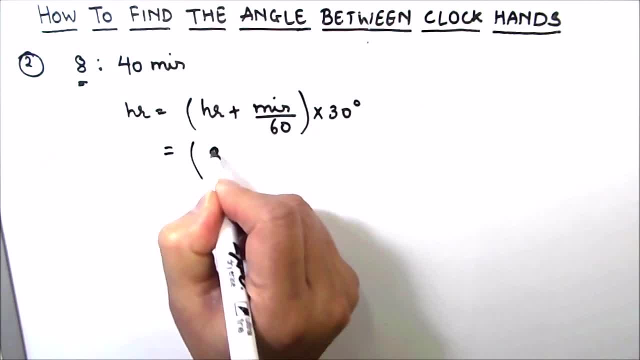 Which is equal to. we have 8 hours here, 8 hours plus 40 minutes. So 40 minutes divided by 60 multiplied by 30 degrees, So this will become 8 hours, 40 minutes. 8 plus 2 by 3, multiplied by 30, which is equal to 26, by 3 multiplied by 30, which is equal. 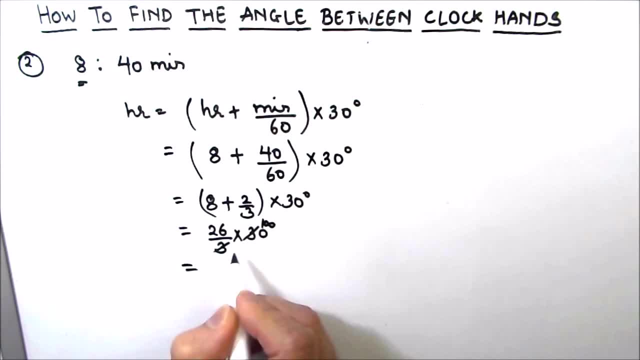 to 3 times 1 and 3 times 10.. This is 260 degrees. Angle made by the hour hand is 260 degrees. Next, we will find the angle made by the minute hand, Which is minutes. Minutes multiplied by 60.. 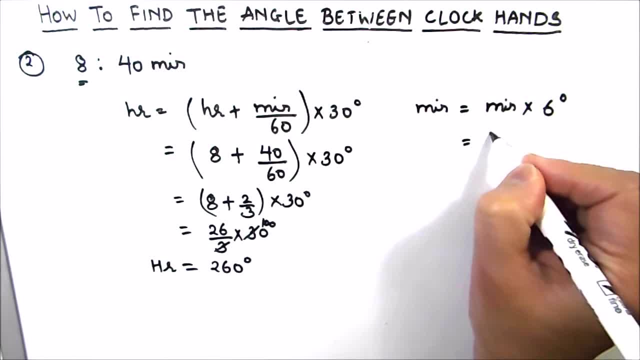 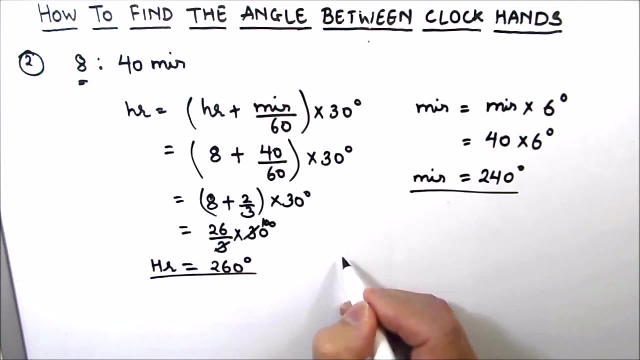 Every minute it is making 60 degree angle. So we have 40 minutes multiplied by 60, which is equal to 240 degrees. So the angle made by minute hand is 240 and angle made by the hour hand is 260.. So the final angle between the hands is equal to the absolute value of the hour minus minute. 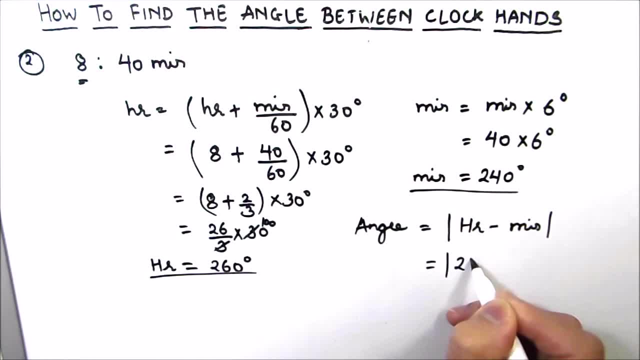 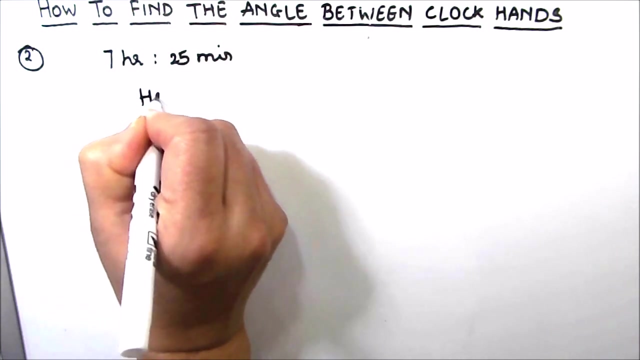 angle. so we have hour angle as 260 degree and minute angle as 240 degree, which is equal to 20 degrees. so the angle made between the hands of the clock when the time is 8 hours 40 minutes is 20 degrees. let's try one more example for 7 hours 25 minutes. so the angle made by the hour hand is: 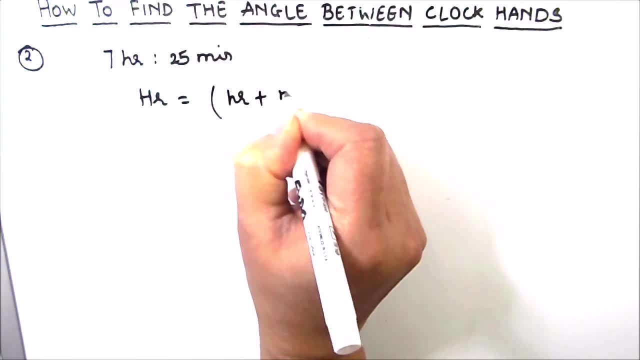 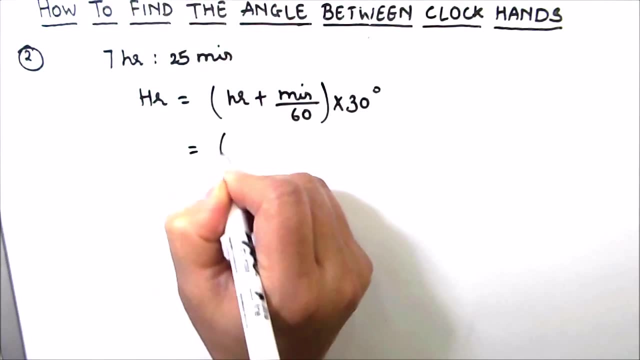 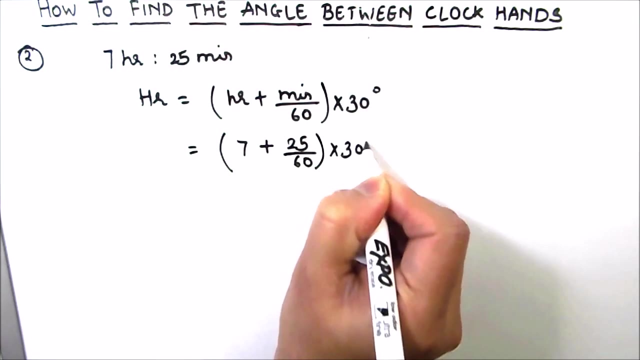 hour plus minute hand divided by 60, multiply by 30 degrees, which is equal to 7. hour plus minute is 25 minutes divided by 60 multiply by 30 degrees. so this is equal to 7 plus 5 times 5 and 5 times 12, 5 by 12. 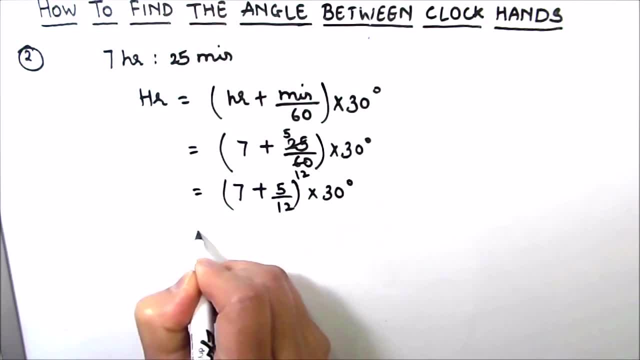 multiply by 30 degrees, which is equal to 12 times 7, is 84 plus 5, divided by 12. multiply by 30, which gives us 89 times 30 degrees. divided by 12, this comes out to be 6 times 2 and 6 times 5, which is equal to 222.5. 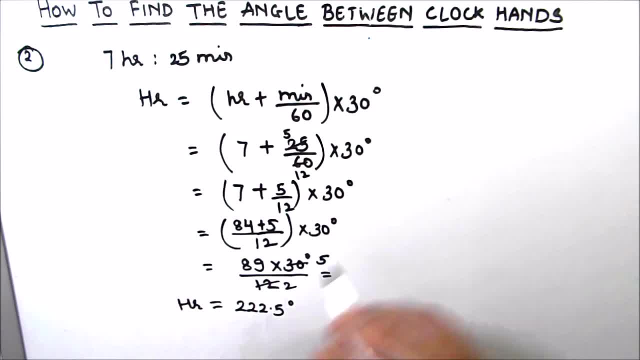 this is the angle made between the hands of the clock when the time is 8 hours, 20 minutes is 20 degrees made by hour hand. now we'll find the angle made by the minute hand. minute hand is minute times 6 degrees, which is equal to 25 times 6 degree, which gives us 150 degrees. so the angle made by the